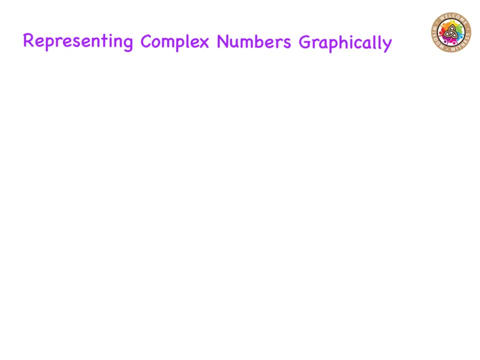 the real number line and, just as we've done lots of times in the past, we can also represent complex numbers graphically. So it's just another type, and the diagram that we use for complex numbers was invented by this guy here, Jean Robert Argand, and he is the one to bring. 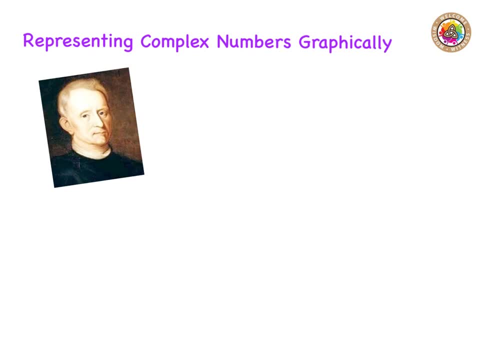 about the kind of plane that we use to represent complex numbers, And it's called the complex plane and after him it is known as the Argand diagram. Okay, so very often we will see plot such and such on an Argand diagram and straight away we'll know we're dealing with. 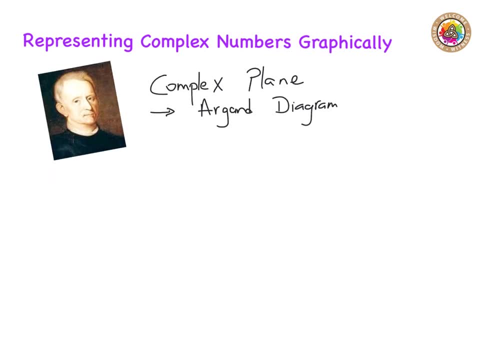 complex numbers. So that's something really important for us to remember. And the Argand diagram looks just like this. So it's made up of two different axes: The real axis for the real numbers and the imaginary axis for the imaginary numbers. So the real axis is along the horizontal axis and the imaginary numbers they go along. 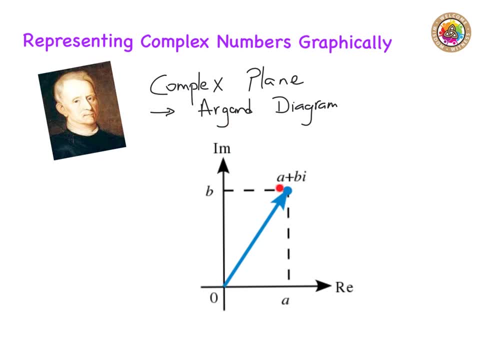 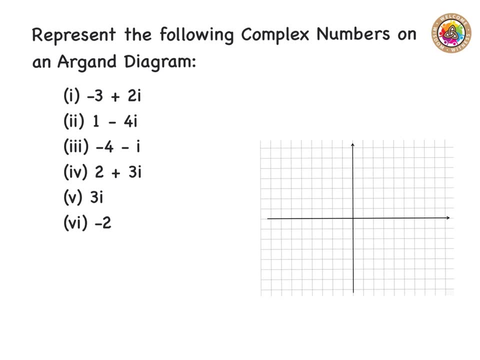 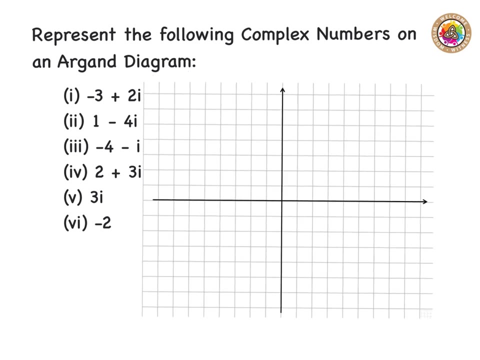 the vertical axis. Okay, so we're just going to simply attempt to represent some complex numbers graphically. Okay, so here we go. we're asked to represent the following complex numbers on an Argand diagram. So the first thing here is I draw my vertical axis and I draw my horizontal axis and I label them. So I know that my horizontal 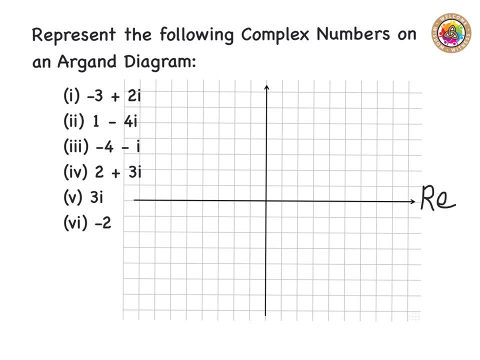 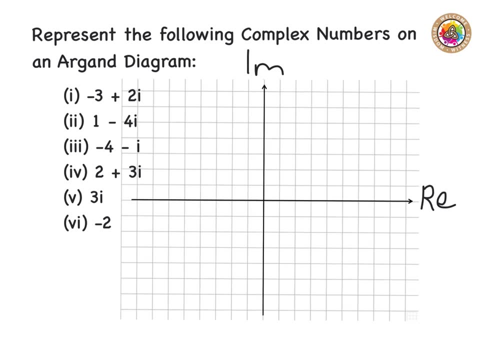 axis is the real axis and my vertical axis is the imaginary axis. Okay, so now that I have those drawn, I also must arrange here the numbers along the horizontal axis. So I'm just going to plot the numbers along my axis. So I'm just going to plot the numbers along my axis. 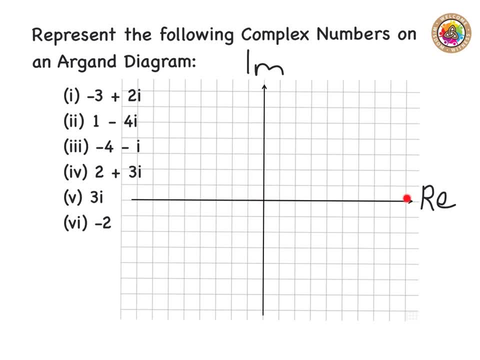 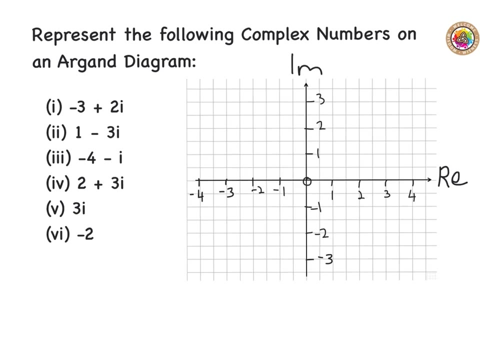 Again remembering to start at zero and to work my way out from zero. Okay, positive, negative, positive, negative, Okay. so I'm just going to plot those very quickly. Okay, so we're going to take the first point here and that's minus 3 plus 2i. So I go to minus 3 on the real axis and I go up to 2 on 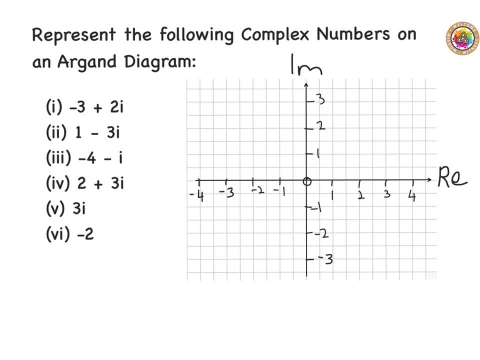 the imaginary axis. And so there we go. I have minus 3 plus 2i right here. Okay now, and I'm just going to mark that off: That's minus 3 plus 2i. Okay now. the next one says 1 minus 3i. So again, I. 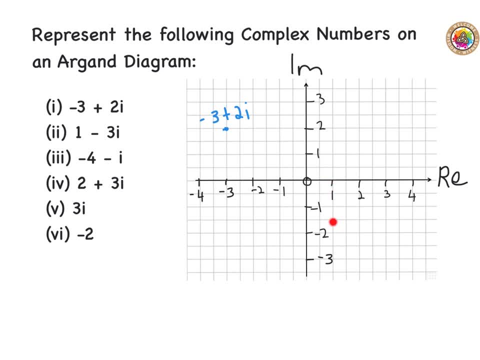 go here to 1 on the real axis and down as far as minus 3 on the imaginary axis. So this point here, that's 1 minus 3i, And again I'm going to mark that in there and I'm going to label it 1 minus 3i. The next one: 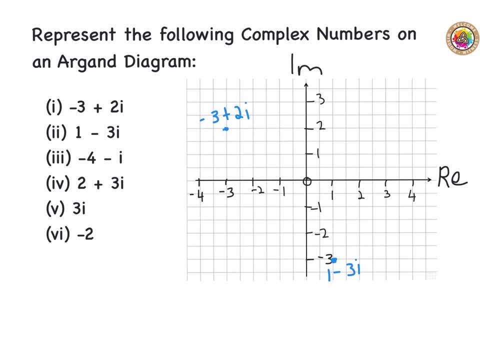 then we're asked: minus 4, minus i. So again I go to minus 4 on the real number line and down as far as well, minus i, I know that's the same as 1i, So or minus 1i. So I go down here to minus 1.. 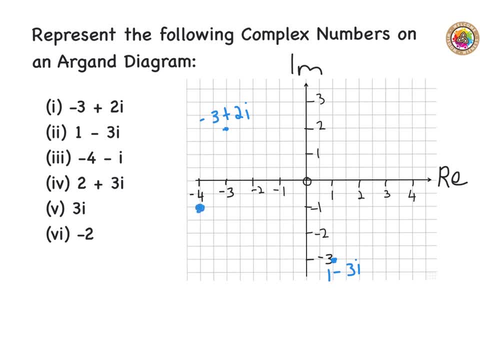 Okay, so I'm going to plot that there. So that's minus 4 minus i. The next one then that we have is 2 plus 3i. So here I'm going to go to 2 on the real number line and up as far as 3 on the imaginary axis. So that's going to be this point. 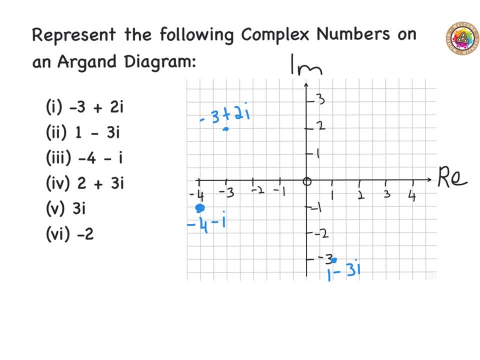 here: 2 plus 3i. And again I'm going to plot that: just here: 2 plus 3i. Now on to. we've a couple of difficult ones here now where we have just one part of the complex number. So the complex number is just, in this case, along the imaginary axis. But I know that. 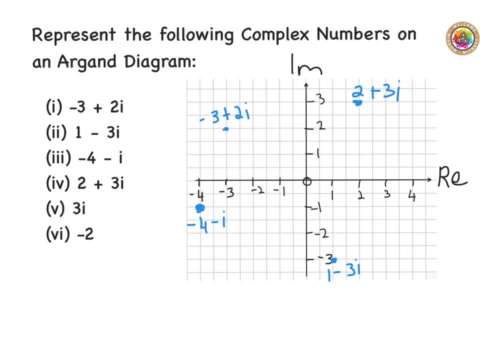 that's the same as when I see just 3i. I know that's the same as 0 plus 3i. So I go to 0 on the real axis and I literally just go straight up to 3 on the imaginary axis And that's going to be. 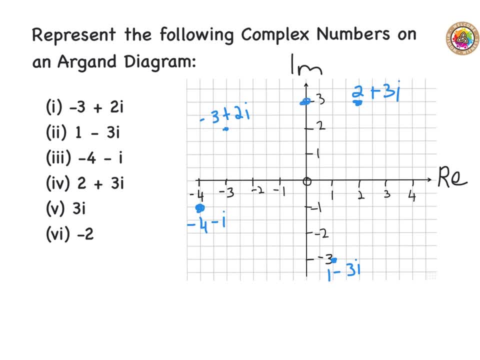 that point there. So I'm going to plot that point there And I'm going to label it 3i. And likewise here for the last one, I have minus 2.. So here I'm going to go. I know again that's minus 2 plus 0i. So I know. 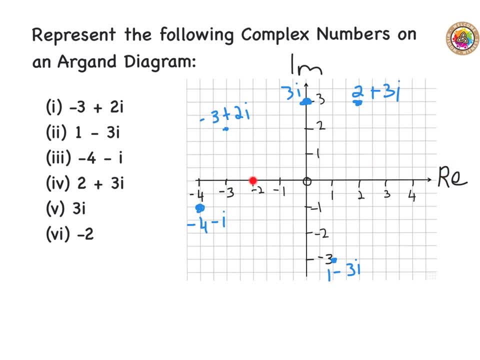 it's just along the real number line, And so here is minus 2 on the reals And I'm going to plot that and label Minus 2.. Okay, So that's pretty much it for the basics on plotting or representing complex numbers on the. 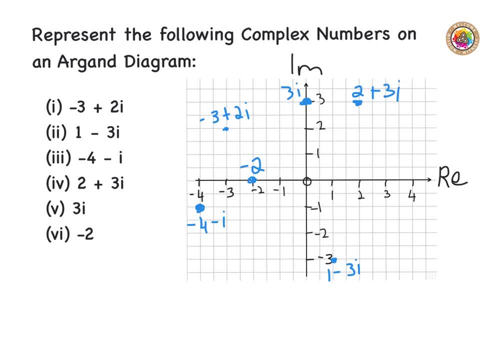 Argand diagram. So if you open up Schoology, you'll be able to see now questions relating to representing complex numbers on the Argand diagram. 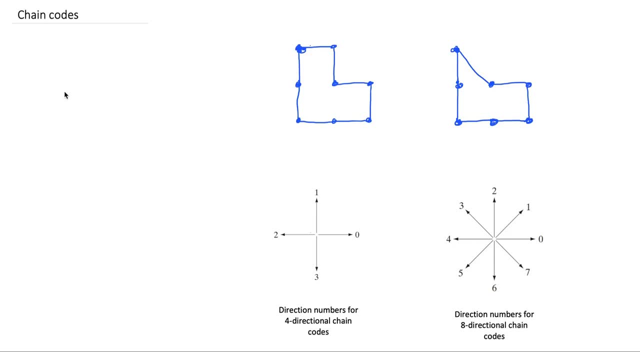 In this video we will talk about the idea of chain codes. So chain codes are basically used for representing a boundary or it is used for boundary 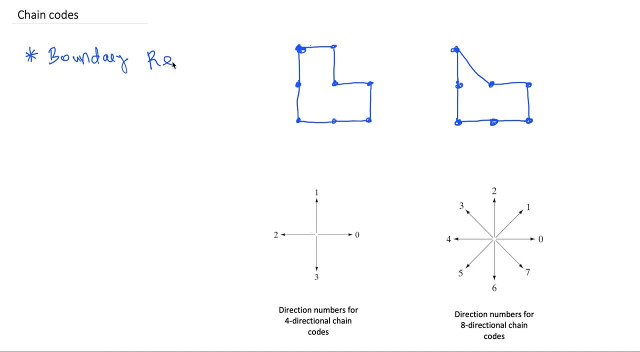 representation. In order to represent a boundary using chain codes we must have the boundary as a sequence of straight line segments of a specific length and 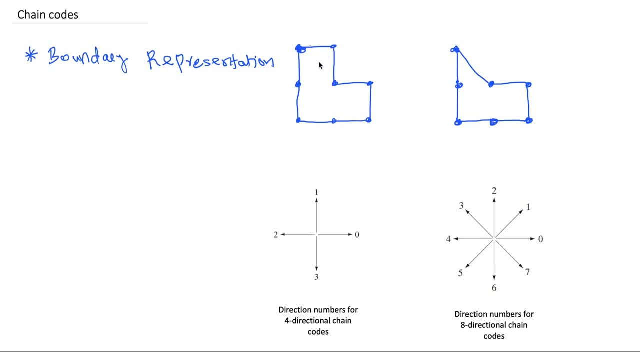 direction. So if you have a boundary formed by the straight line segments of a specific length and direction then you can use chain codes to represent that